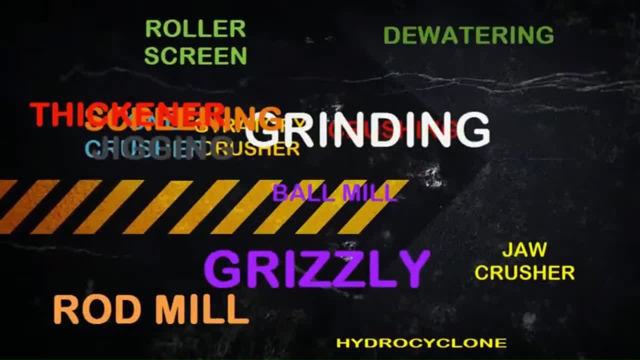 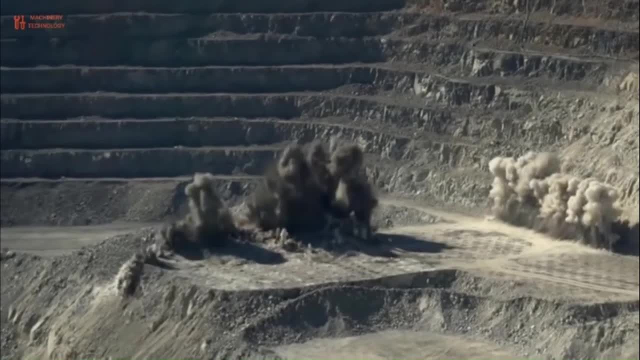 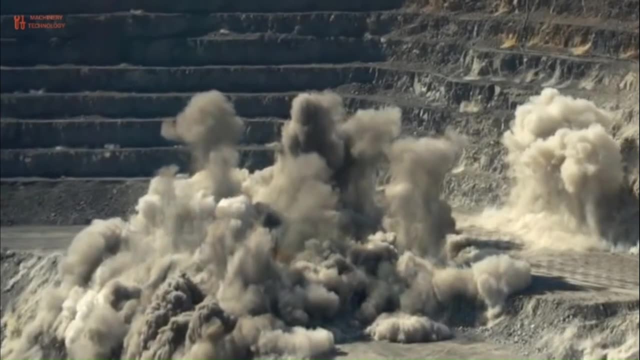 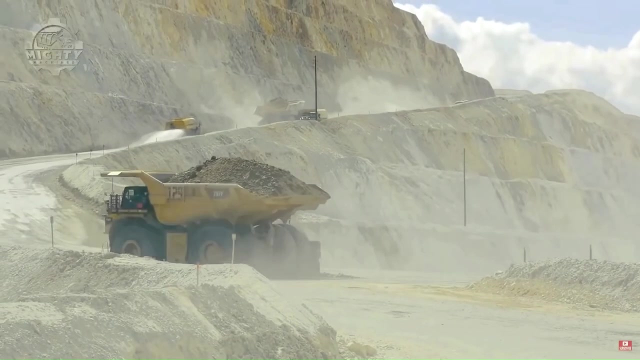 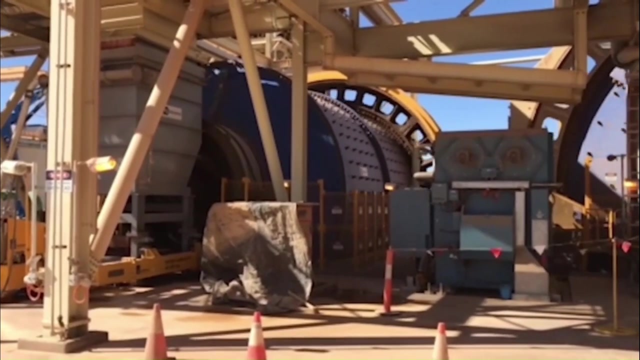 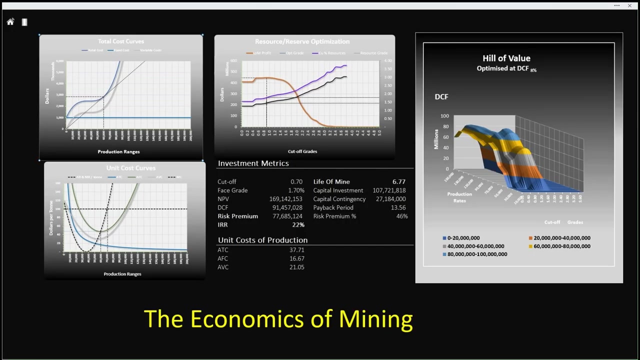 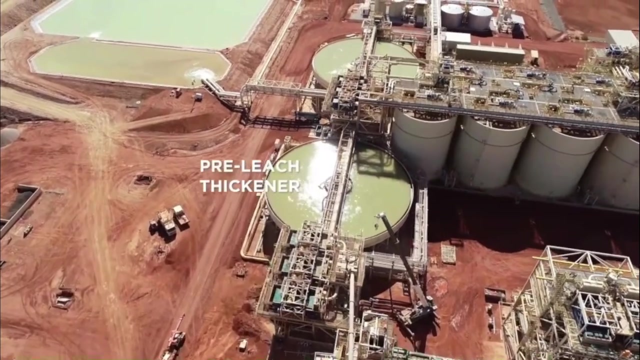 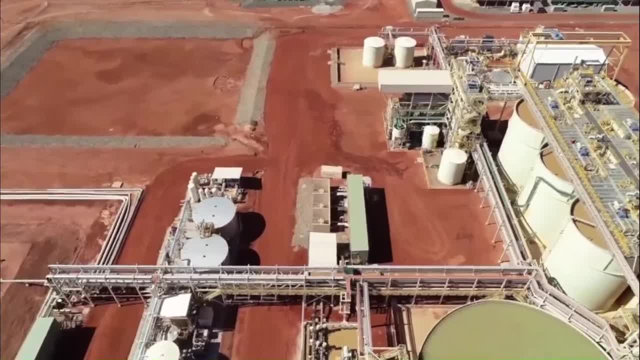 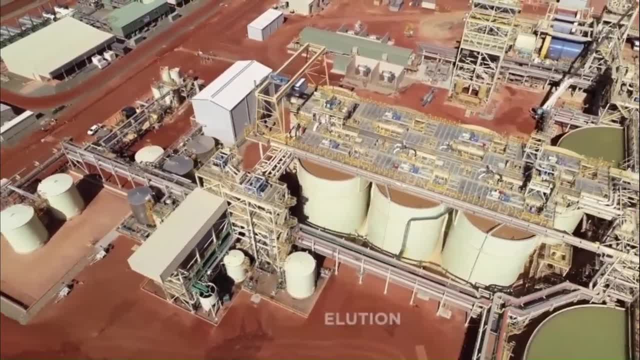 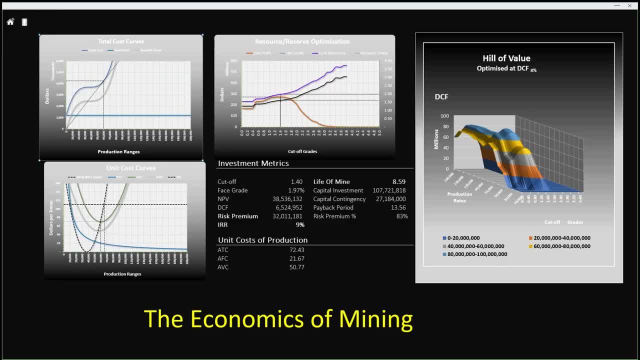 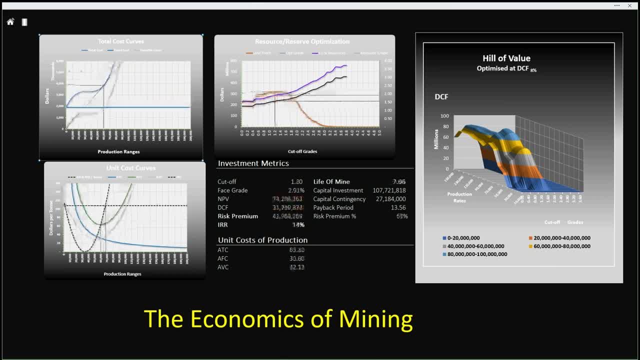 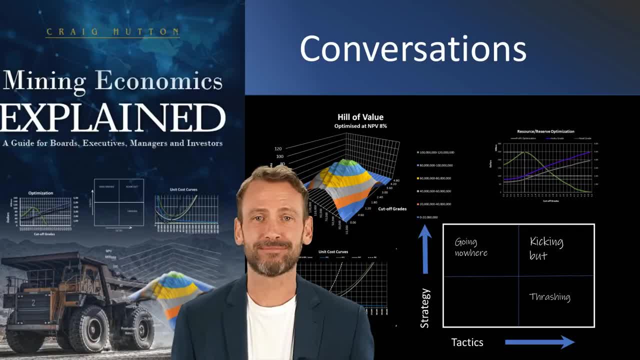 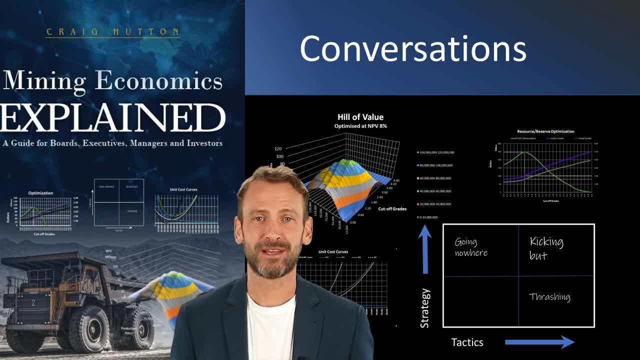 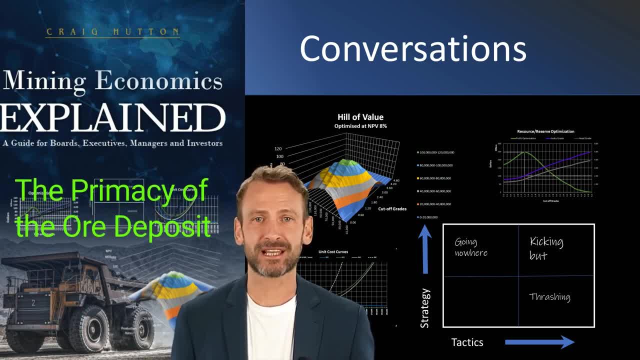 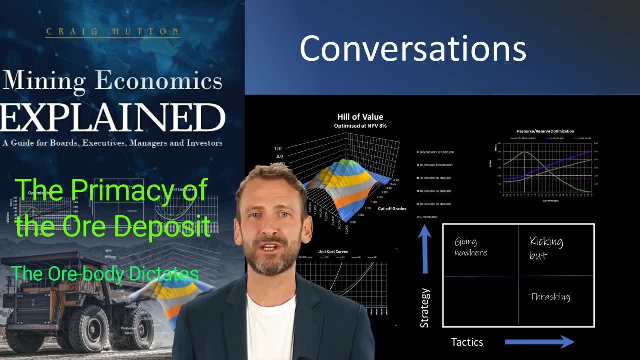 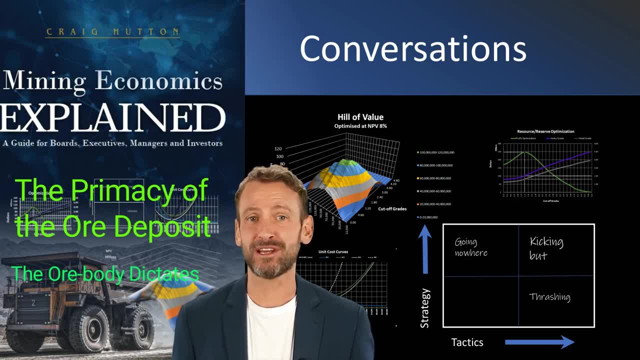 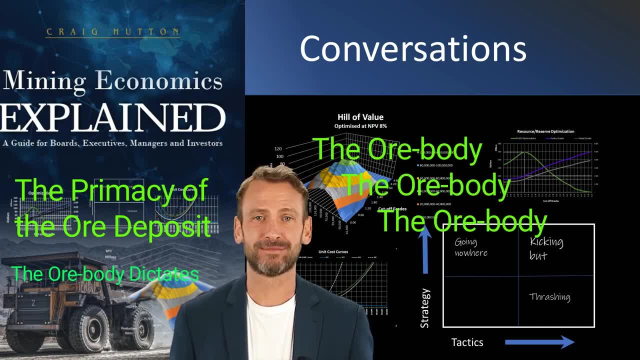 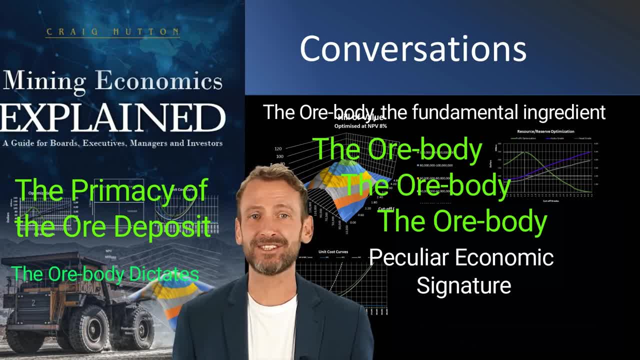 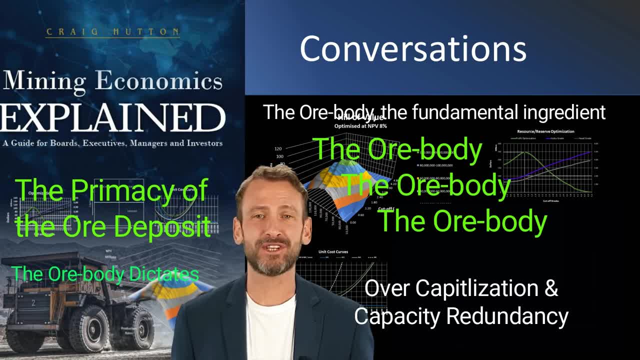 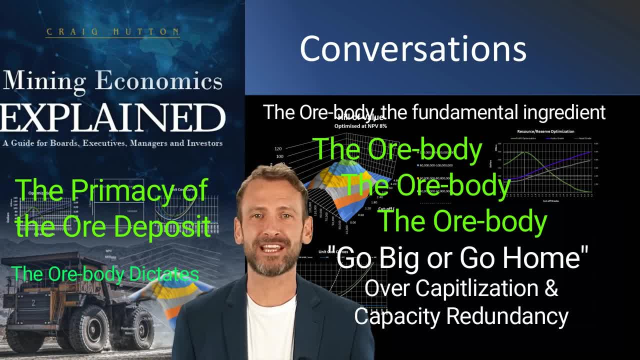 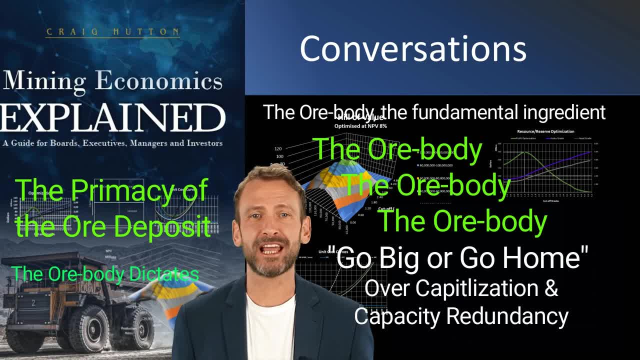 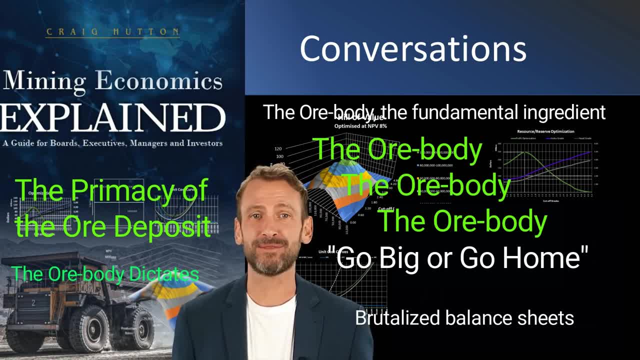 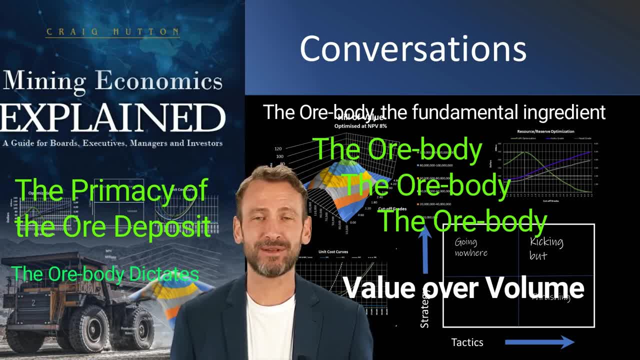 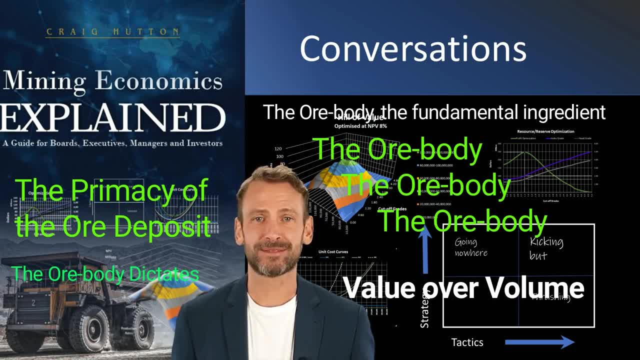 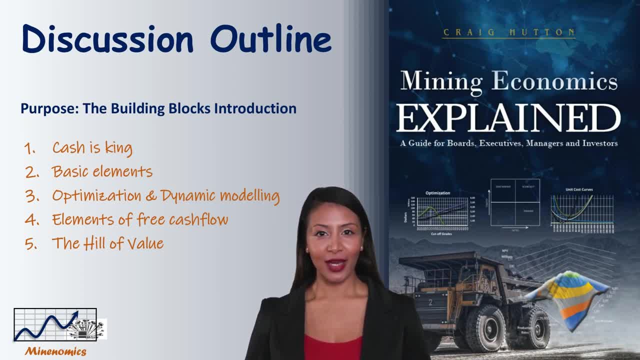 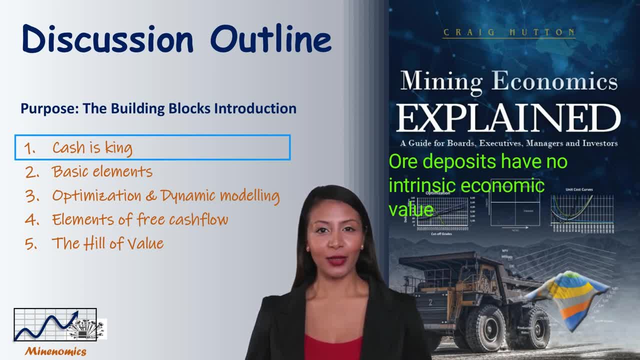 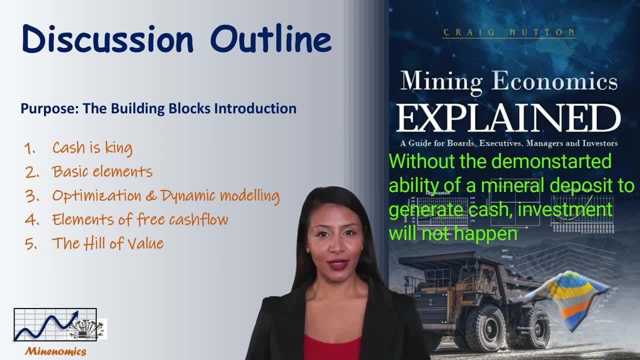 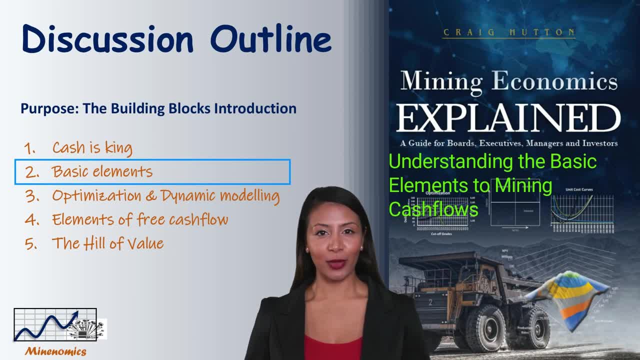 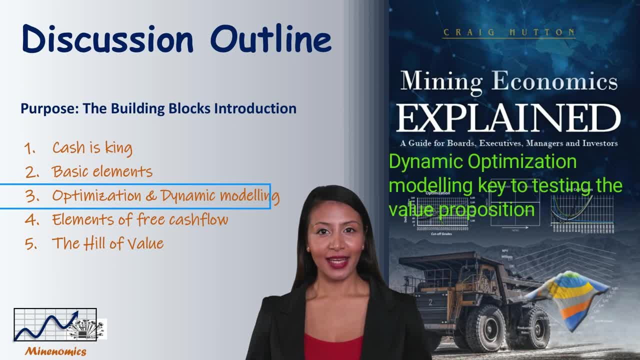 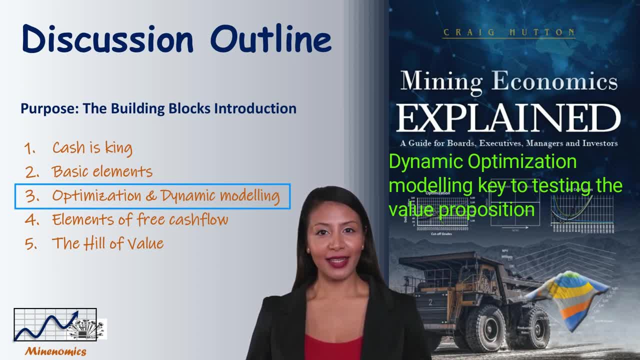 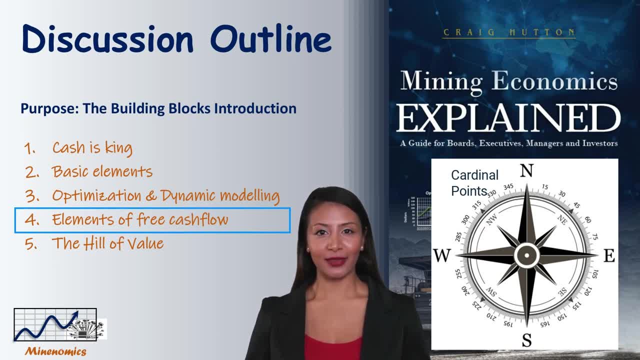 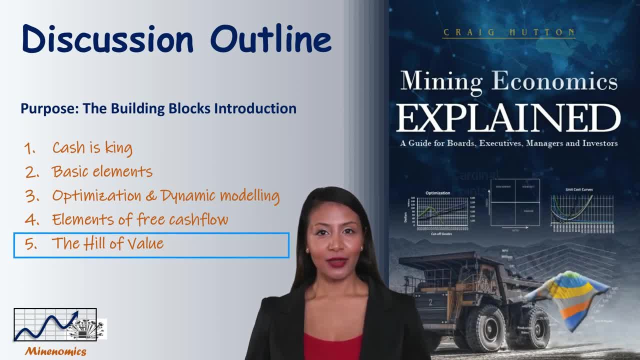 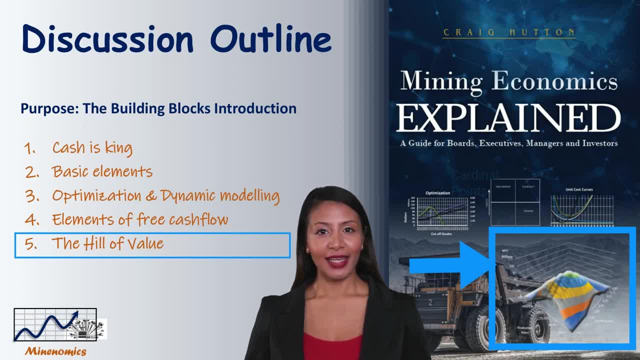 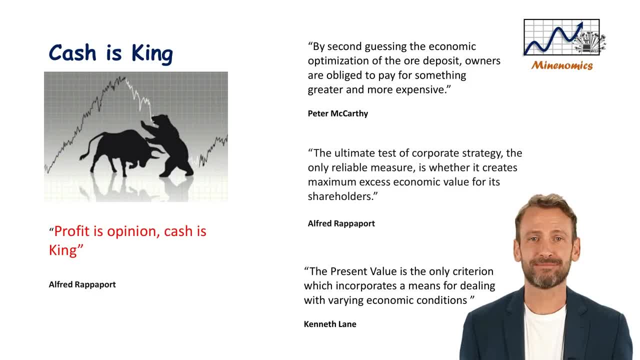 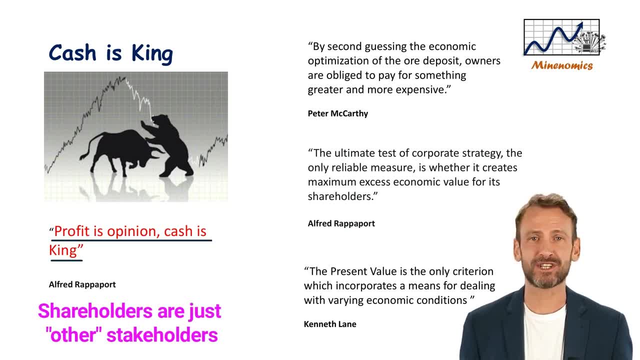 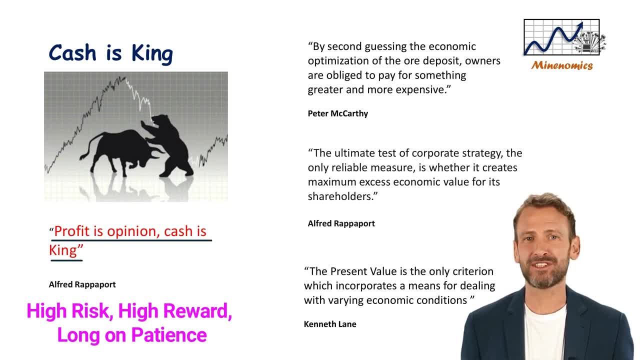 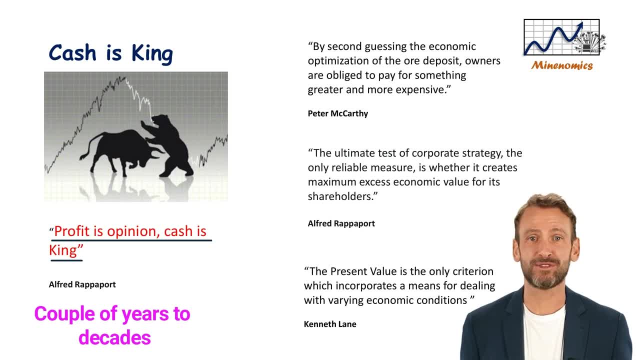 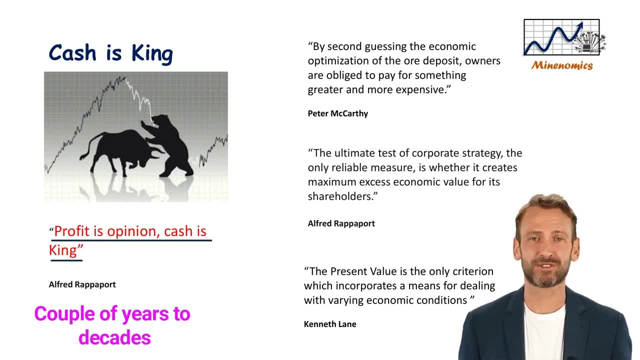 Thank you very much for watching is made to when the first dividend check arrives. significant risks and uncertainties must be contended with, namely: price volatility, commodity cycles, taxation and royalty regime uncertainties, nationalization and free-carry equity grabs, inflation, supply chain disruptions. 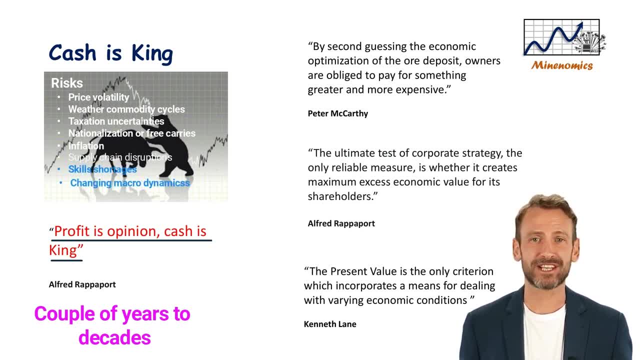 skills shortages and changing macro-dynamics, to name but a few. Alfred Rappaport said that in order to reward these high-risk, high-reward patient investors, it is required to create maximum excess economic value for shareholders. This, in his view, is the true test of corporate strategy and the only reliable measure of success. 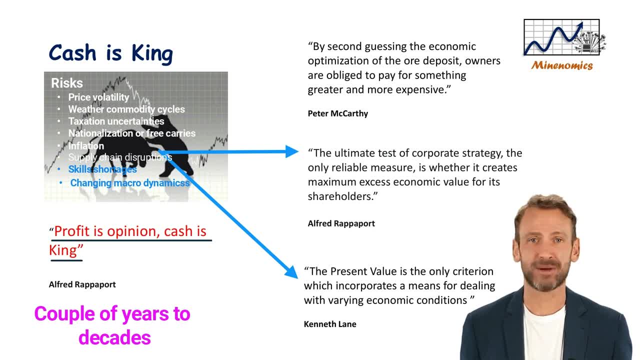 To achieve this, an ore deposit must be optimized to maximize the net present value that a peculiar deposit can yield. Many a mine fails because management seconds. Second guess is the optimization of the ore deposit. As a result, owners are often forced to pay for something greater and more expensive. 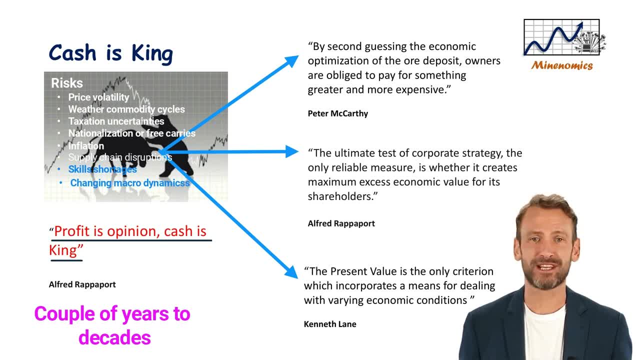 because the operators have a poor comprehension of economics. Craig's mantra to management is: plan your flight, fly your plan. As we unpack the tools needed, an emphasis will also be put on demonstrating how management teams have the tools to not only optimize their deposits but track their performance. 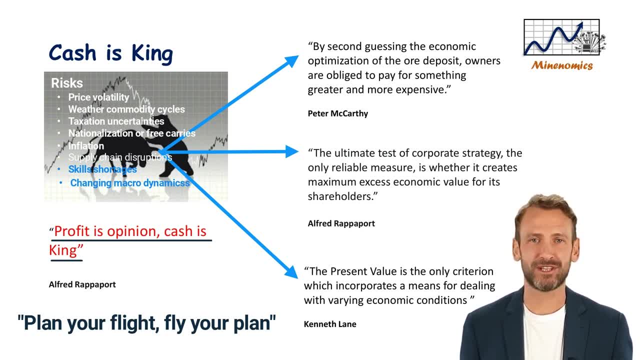 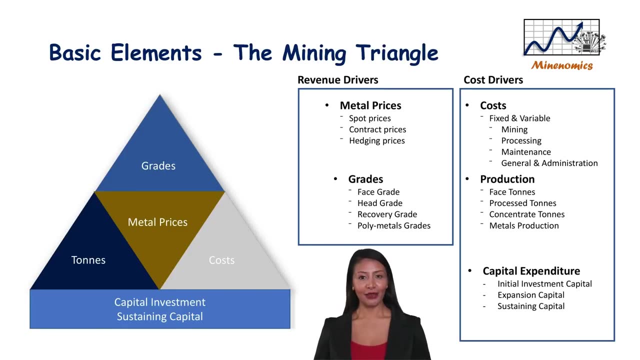 against the odds. If managers fail to do this, investors today will punish management. Before we get there, let's look at some basic concepts that underpin mine optimization. The basic elements related to mining cash flows are neatly summarized by the mining triangle. 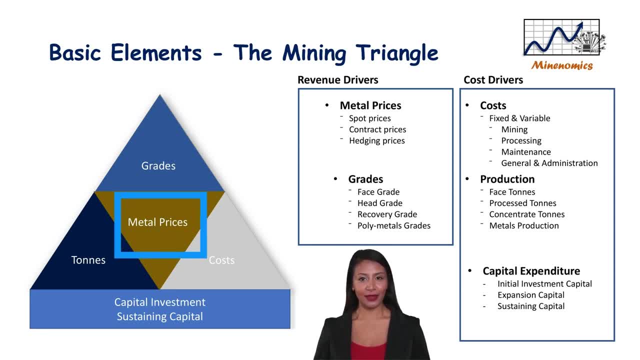 The first element is the metal price or prices. The metal price or prices assumed are the single most impactful variable on net present value. The price assumptions adopted are key to mine optimization. ergo, we will spend some time in a later video discussing this important topic. 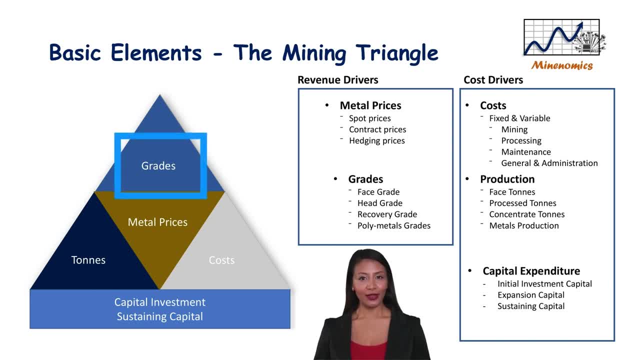 The second is grade. There are various grades that need to be understood, because metal grades have an equally impactful result on the net present value calculation. We will spend more time on this topic when we unpack the formulation of the basic mining equation. The third is cost. 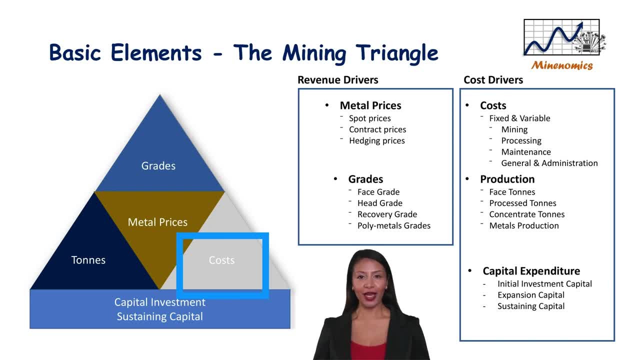 Microeconomics defined the concept of fixed and variable costs. Whilst this concept is well embedded in the thinking of miners, the modeling of these costs is poorly done. We will dedicate much time to discussing this concept and its application, as it is a major component of the optimization algorithm described in mining economics explained. 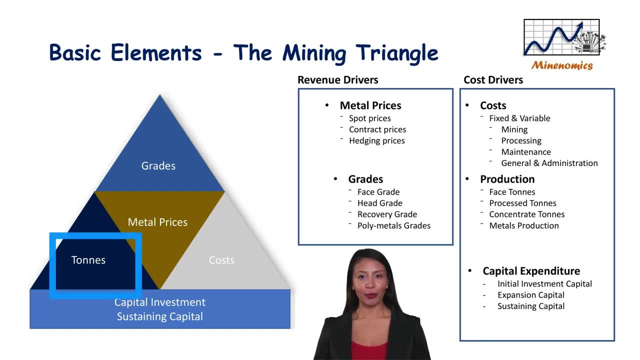 Fourth, production. Mining is peculiar in that production is not defined by the product produced. Rather, it is defined by the volumes of tons that are moved and processed. Tons mined and processed drive costs rather than the metals produced. The metals produced drive revenue. 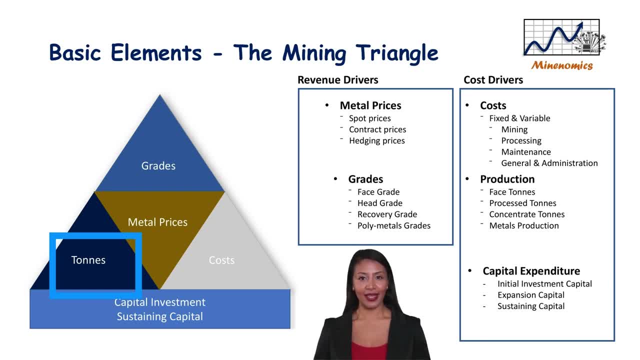 This is a cardinal concept to grasp and fundamental to mining economics. Fifth, capital investment. In order to establish a mine, a significant capital investment is required. Moreover, when that investment has been made and the mine has been established, there is an ongoing investment requirement, commonly referred to as sustaining capital. 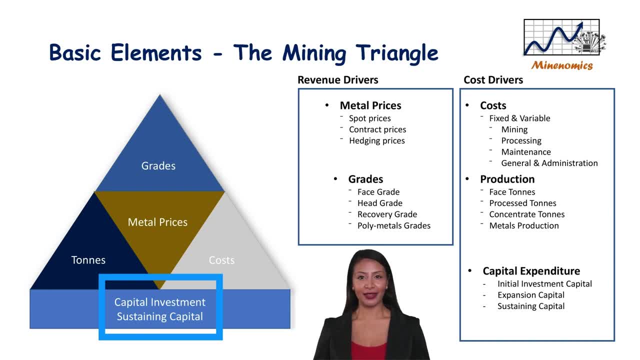 This is the investment that management teams must realize superior returns on. If they do not, that money will be invested elsewhere, in alternative projects that will yield higher returns. A key message here is: tons drives costs, Grades drive revenue. Grade always trumps scale because of this. 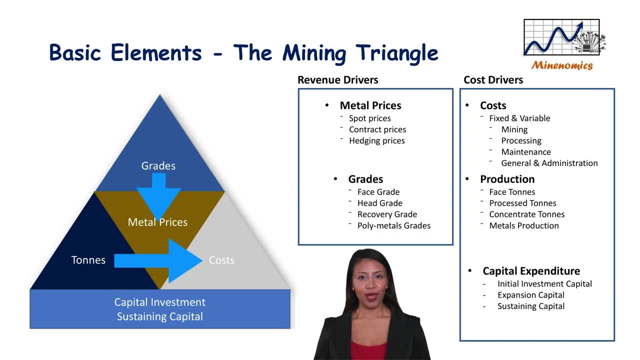 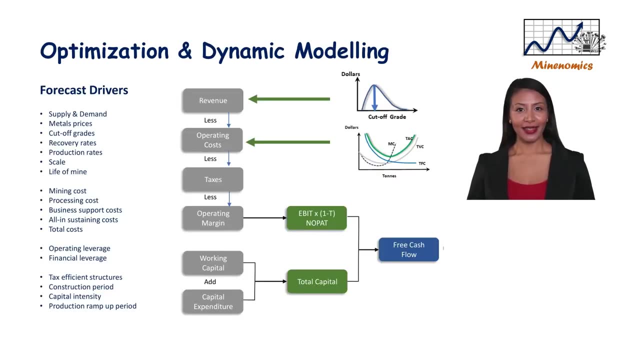 Smaller, higher-grade mines will always outperform low-grade mines. Smaller, higher-grade mines will always outperform low-grade mines. High-grade mines are also extremely useful in a greater mining company's overall portfolio. for the same reason, As Jason has pointed out, it is essential to maximize returns for shareholders. 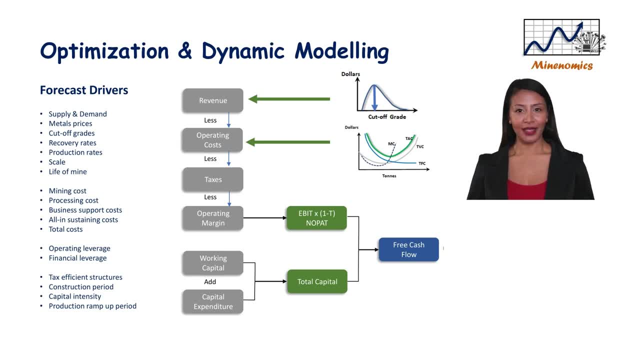 If maximum returns are not prioritized, then an opportunity cost is incurred. An opportunity cost is the return on investment foregone When compared to another investment. mining companies compete in capital markets and therefore understanding how to maximize returns for a mining project is the fundamental mission of mining economics. 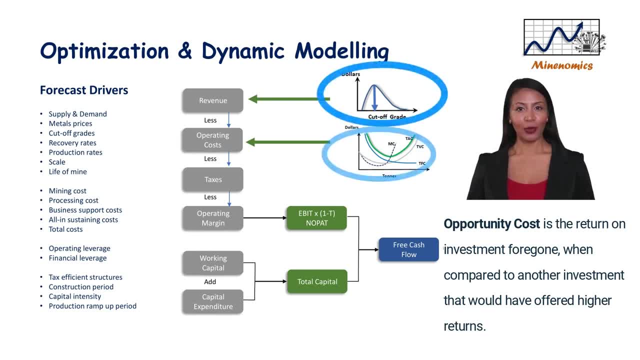 To do this, we have to optimize the cut-off grade and the optimal production rate or scale of operations to minimize operating costs and maximize profitability. This requires comprehensive, dynamic modeling of a myriad of assumptions, technical and economic. as outlined in this slide, Multiple cash flow profiles can be generated for a single deposit. 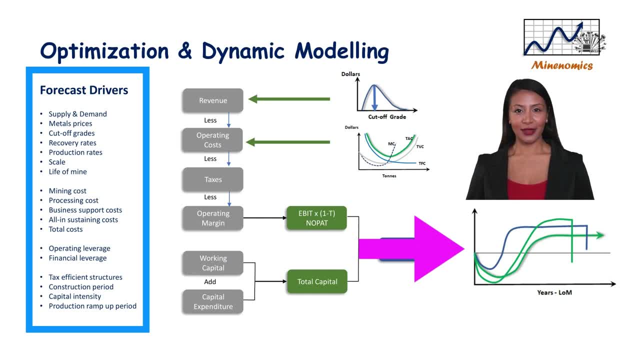 based on the mining and processing path selected. The trick is to discover the mining and processing path that maximizes cash flows for a given ore body. To do this, we have to model the ore deposit and make a myriad of assumptions, technical and economic, as outlined in this slide. 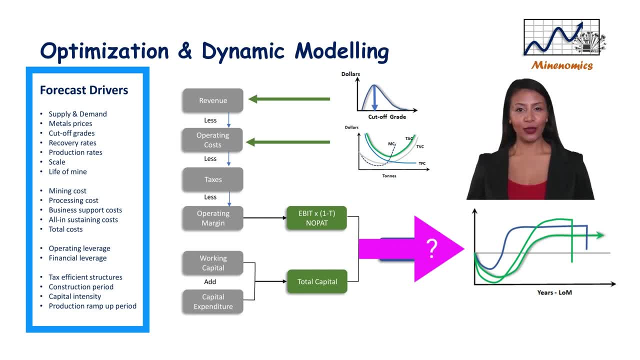 To achieve this, we have to understand the sweet spot of a peculiar ore body. By determining the cut-off grade of a deposit and the optimal economic costs to produce at, and by taking into account all the value drivers, we can estimate the maximum discounted cash flow. 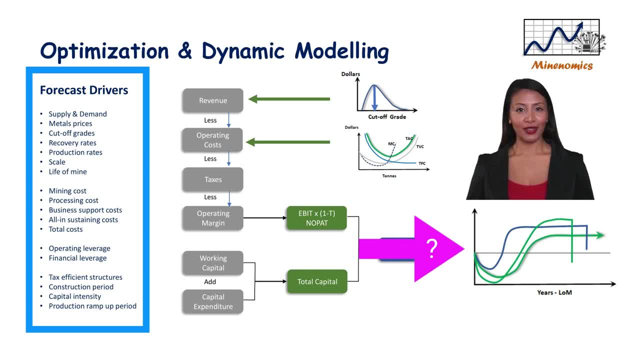 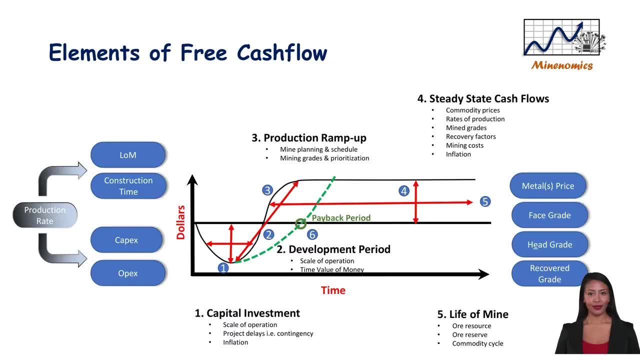 that we can reasonably expect. Before we explore this, let's first consider key elements we need to consider in an optimization algorithm. There are six elements to the cash flow profile that we need to be conscious of when maximizing cash flows. The first is the quantum investment. 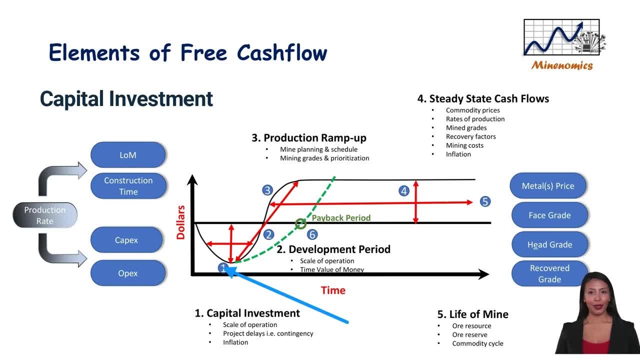 required. The greater the investment, the lower the net present value. The key elements driving the initial investment are primarily the scale of operations and the complexity of the operations. The bigger the investment, the bigger the contingency allowance. Ergo finding the right. 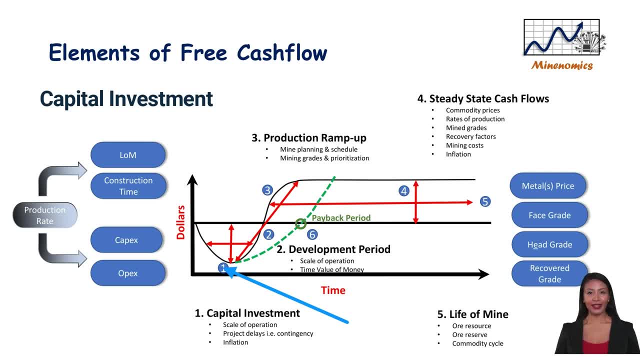 size shoe is a critical optimization element for maximizing the net present value. The second element to the cash flow profile is Приветing the cash flow proposal, The rotations of the все 말�i have an starting MCVs value so that will keep our cash flow. 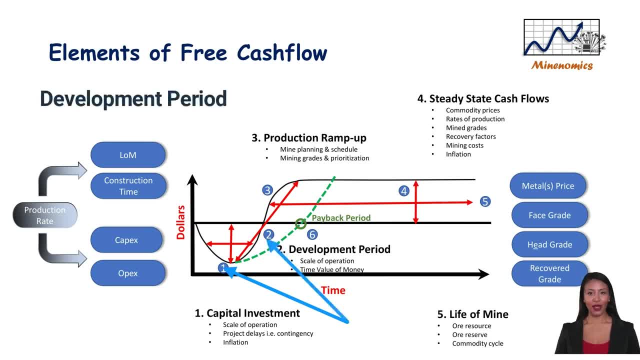 element and as an axiom: the larger the footprint, the longer it will take to build the required infrastructure. Net present value embeds the idea of the time value of money. As a result, the longer things take to build, the more harm to the value of that money expressed as a lower net. 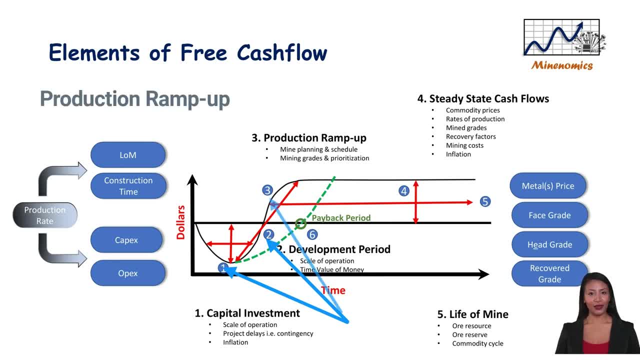 present value. The third element: once the infrastructure has been built, the mind has to ramp up production to a steady state. The larger the footprint and scale, the longer the time needed to reach steady state. production Time is money and the longer it takes to sell. 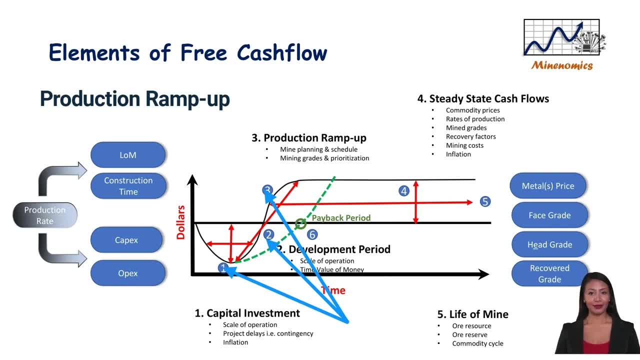 metals, the net present value is negatively impacted. There are many reasons that can retard the reaching the steady state production, For example, in underground mines it depends on the rate of development that can be achieved. in an open pit mine it may depend on the equipment. 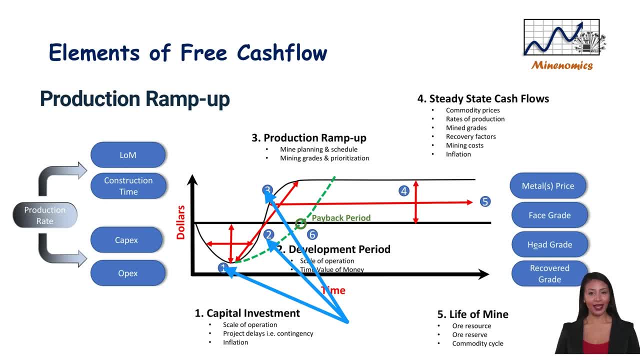 matching The processing plant is also a key player in the ramp-up equation, and the size and complexity of this infrastructure can play a detrimental role. The fourth component is the steady state production level. This is the level that all the infrastructure is nameplated, or the maximum production design capacity, Determining the 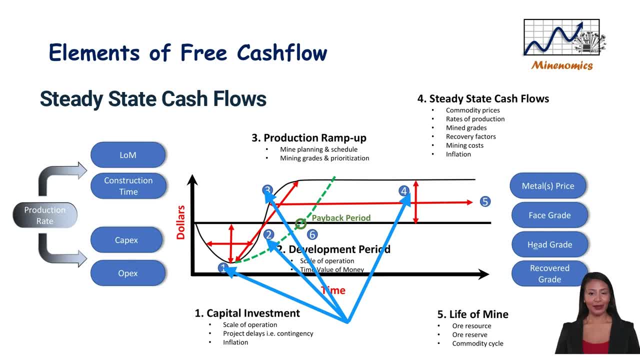 nameplate. production rate is a key optimization parameter that needs to be optimized against the ore body's economic capacity. This is an important aspect of allowing the ore body to dictate and will be a key focus area in subsequent conversations. The fifth component is what is? 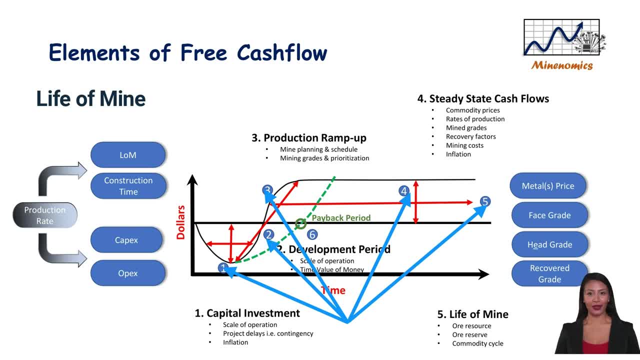 determined the life of mine. Miners can estimate the life of mine by dividing the defined mineral resource by the rate of production. A key optimization is to consider the maximum value by trading off the life of mine against the scale of production. The sixth and final component is the 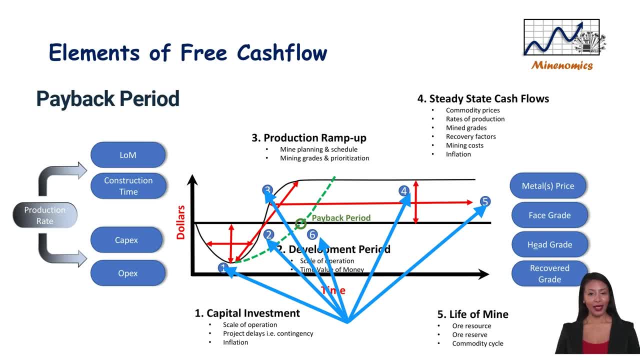 payback period. Investors should be preoccupied by the payback period because it indicates how long it will take for them to retire their risk exposure. Once the payback has been required, investors then seek to be responsible for the production of the ore body. This is a key optimization parameter that 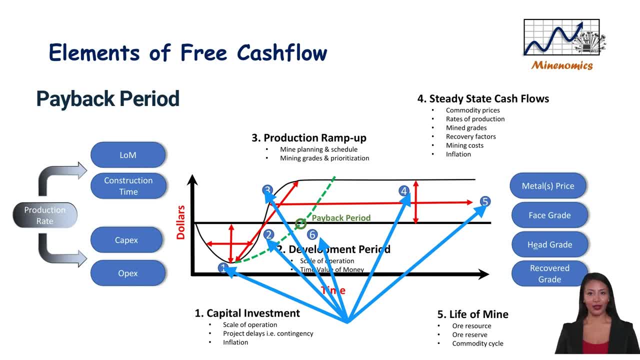 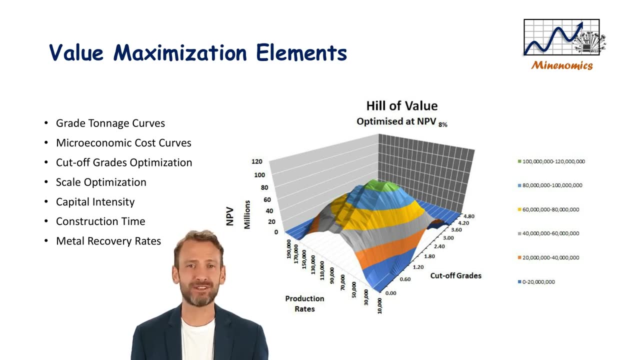 will be rewarded with the return period. The longer the return period, the higher net net present value, and the higher the net present value, the more incentivized the investor will be to invest. Great job, Maya. All the concepts that we have talked about so far need to find their way into. 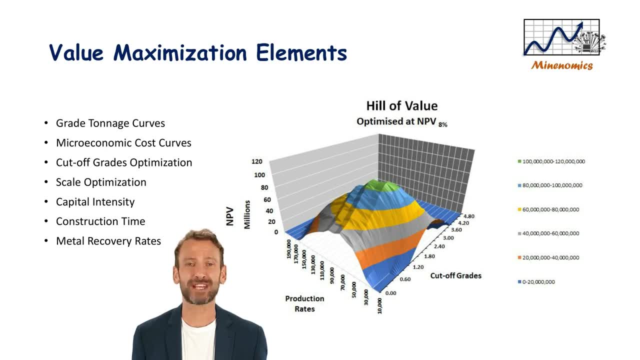 a model that dynamically tests all the variables simultaneously and systematically. We also need to be able to simplistically represent the output. The hill of value is the hill of value. The hill of value is a great way to visualize an optimized solution. This was first conceptualized. 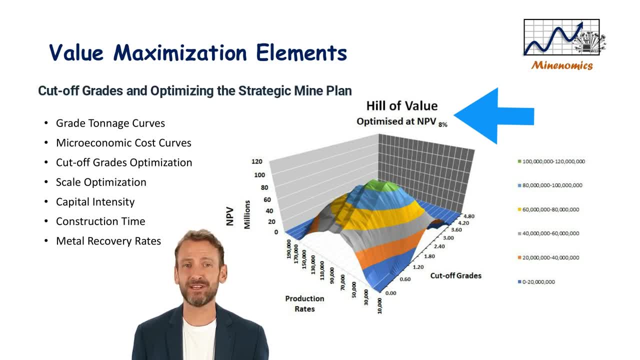 and proposed by Brian Hall and described in his book Cutoff Grades and Optimizing the Strategic Mine Plan. This visualization, the hill of value- has become a useful tool to represent two key decision variables, namely the rate of production and the cutoff grade to be applied to the ore. 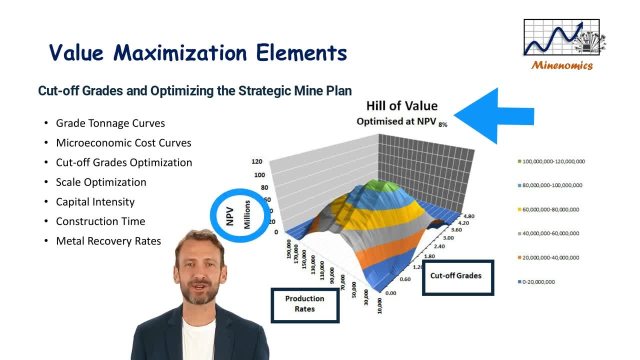 deposit set against net present value. This representation allows investors to be able to determine the optimal rate of production and cutoff grade that will maximize the discounted free cash. To generate a hill of value, a dynamic cash flow model is required that combines an ore deposit's grade tonnage curve welded together with microeconomic cost curves. This is achieved by the 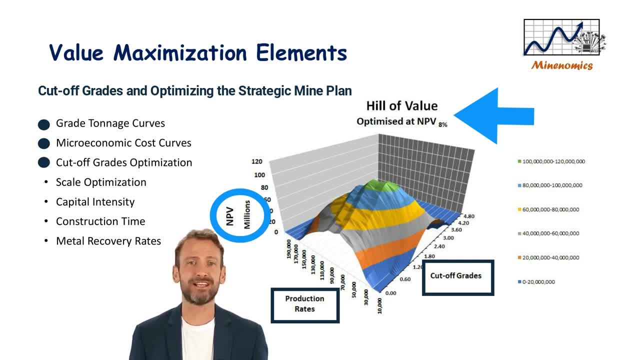 design of a cutoff grade algorithm integrated with a scaling cost curve algorithm. These two algorithms also need to dynamically recognize varying cost curves. This is a great way to understand how anNG 썪y is being built. To understand the cost curve, we need to identify the cost factor which is generated by the 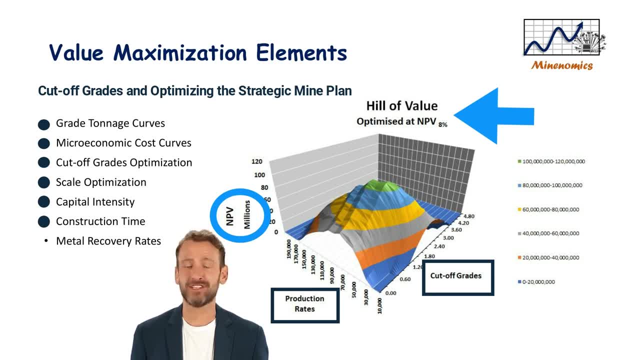 rate of production and cost loss, and then we can distribute the cost to the runoff. The cost factor is a very effective tool to determine the cost of production and cost loss. However, this is also a very useful tool to detect and measure the cost factor. 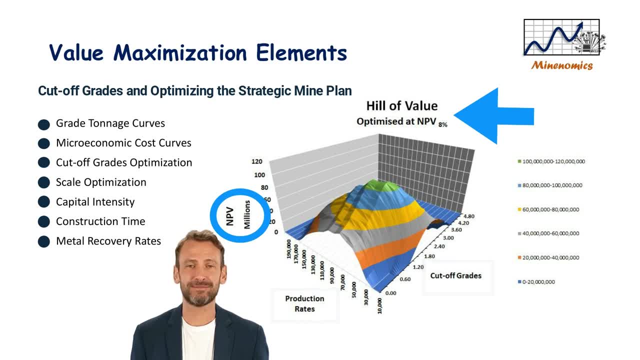 ün. Fundamentally, the lower the cutoff grade, the lower the head grades and the lower the head grades, the lower the metal recovery rate in the plant. Modeling this, we need to understand the costs of current production and cost loss by lowering the cost factor. Indeedters are a number of interesting fundamental factors to consider. The cost of construction is the most important factor. Mercy and cost are both important factors in the development of a flat plant: The cost of complete assay engineering, the cost of preparing and building a metallic 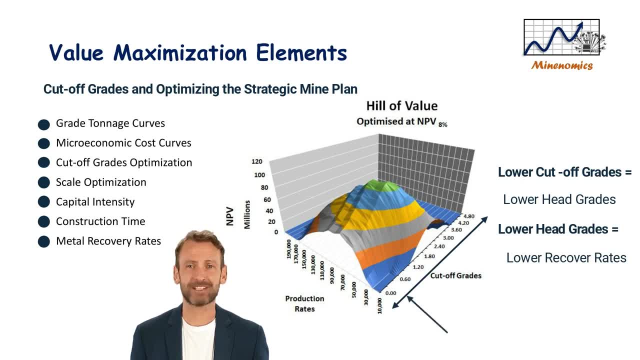 ensures that cut-off grades on the low end realistically reflect reality. Fundamentally, it inhibits cut-off grades that would typically be set too low by management, only to be penalized by lower recoveries. Moreover, lower cut-off grades also perversely incentivize bigger footprints. 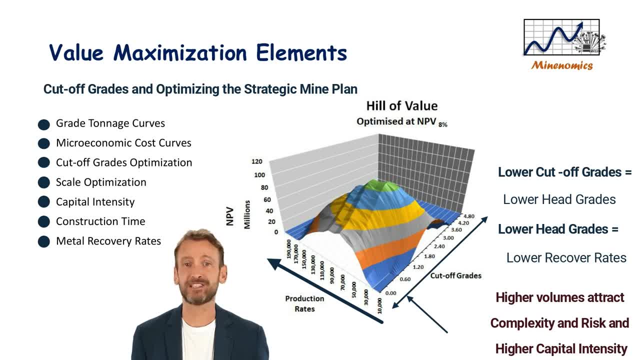 Bigger footprints, are more complex and therefore attract greater risk and greater capital intensity. We will now spend more time looking at each of these concepts and consider how we construct and integrate into a comprehensive, dynamic model that ensures that the ore body dictates decision-making. 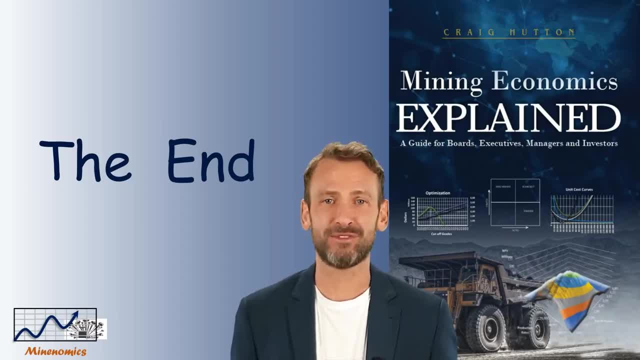 I trust that this video has been informative and helpful, and I invite you to continue our journey by watching more of the videos that follow.